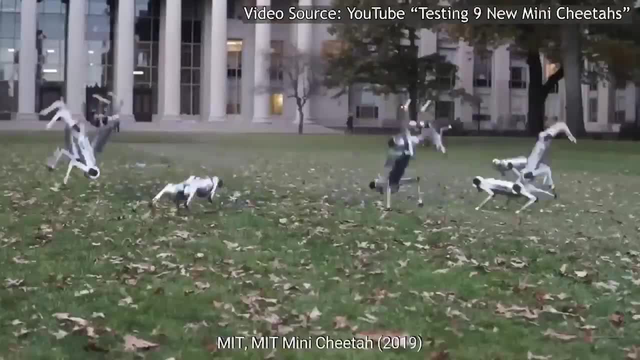 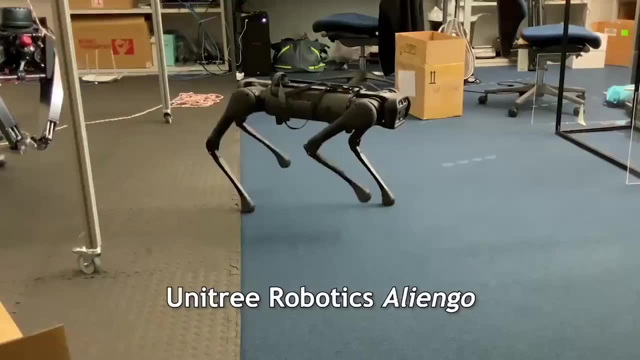 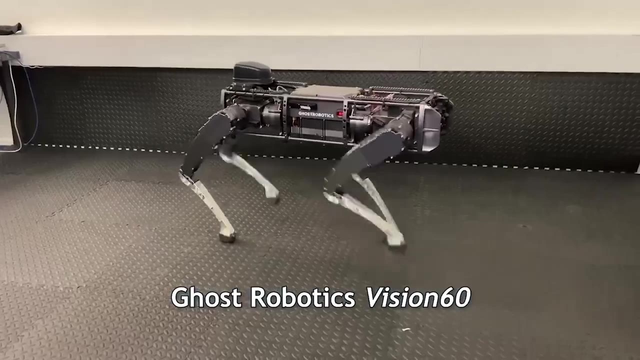 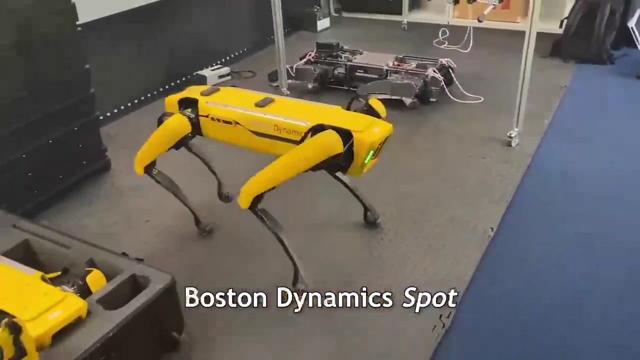 dynamic and agile motions such as running, jumping, backflips, side flips and even dancing. Nevertheless, their movements are arguably stiff and lack the subtle nuances that can easily be observed in animals, As you can see in this video during typical locomotion tasks. 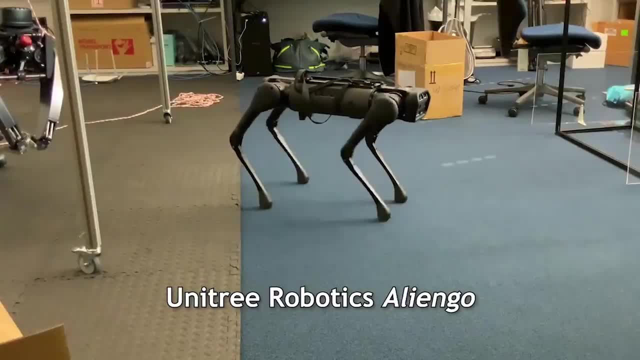 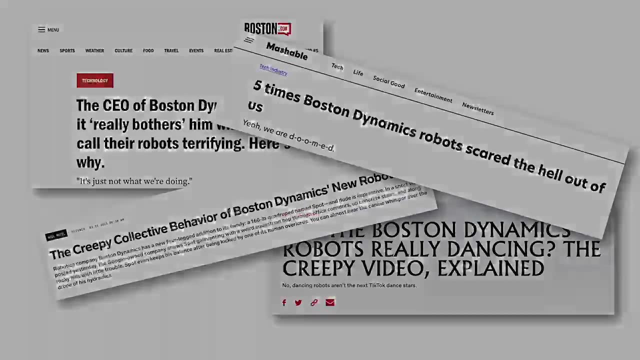 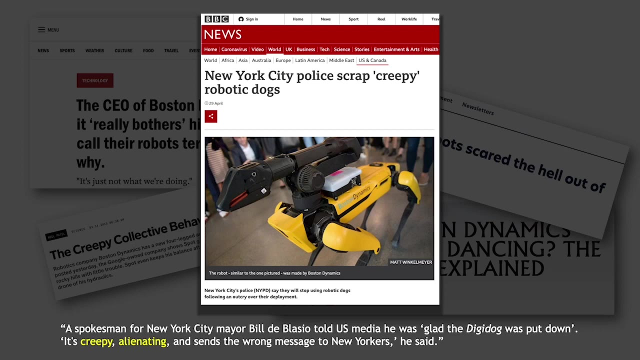 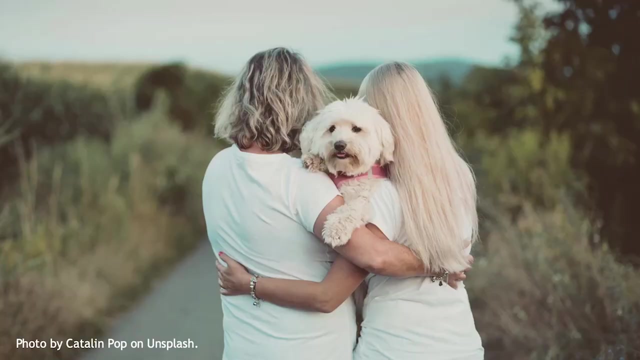 most commercial quadrupedal robots today tend to follow unnatural, asymmetric and regular movement patterns. Such motion features can make robots appear stereotypically lifeless and mechanical and consequently we humans do not feel comfortable in the presence of the robots. Meanwhile, people like dogs. We perceive dogs. 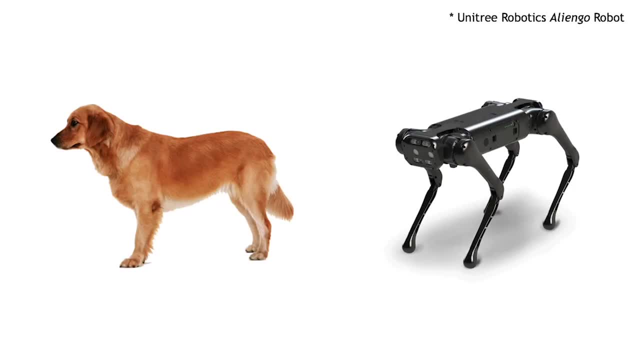 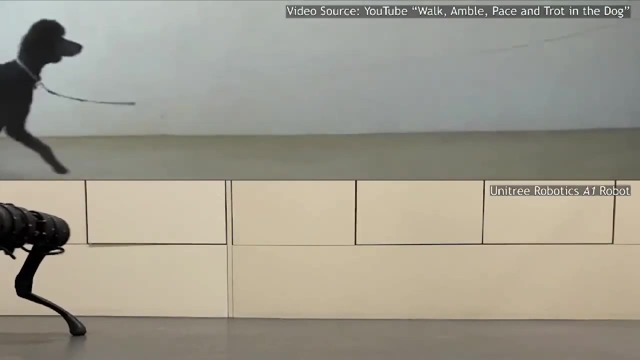 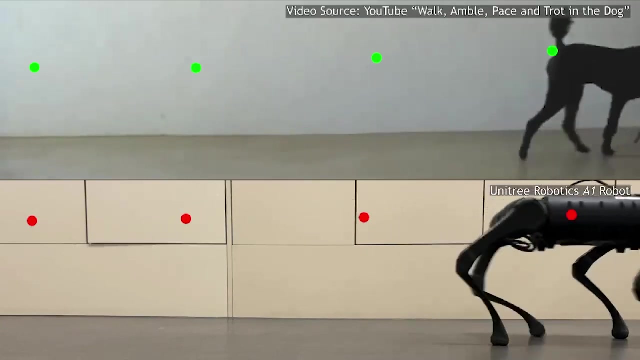 as friendly and relatable. Quadrupedal robots are created with inspiration from their natural counterparts. Their morphology resembles dogs. However, legged robots do not move like dogs. Robots merely persist pre-designed repetitive motion patterns. Due to such a disparity, people still perceive these robots as artificial machines. 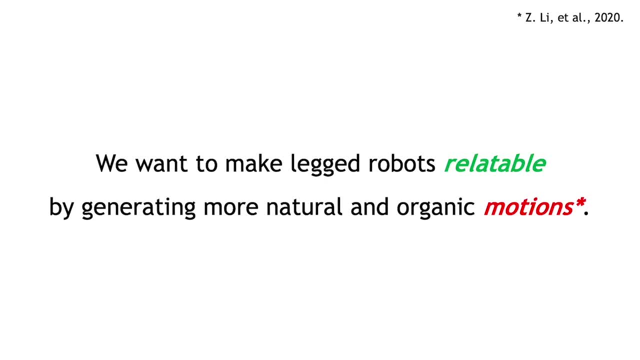 The ultimate goal of this work is to make robots seem more relatable through their behavior. Consequently, we seek to adjust the motions of robots. More specifically, we explore the challenge of generating animal-like walking motions of quadrupedal robots. By doing so, we believe that we can make robots to appear to be living beings. 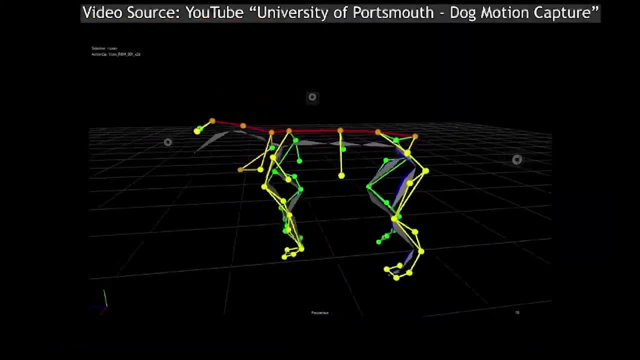 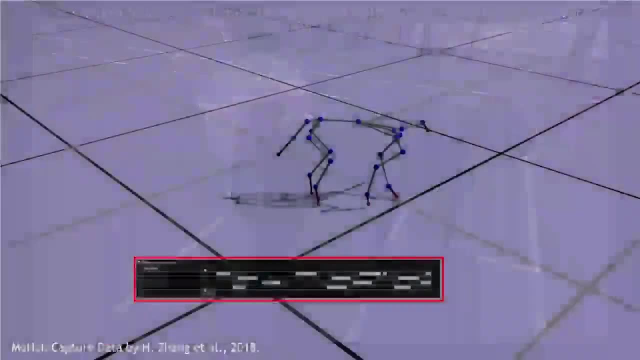 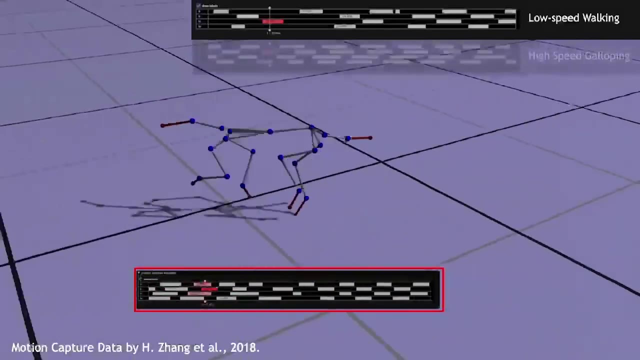 So what is the secret of dogs' movement? We observed a dog's walking motions and identified their main characteristics. This video clip here is a recording of motion capture data of a dog and, as you can see, the dog adopts its walking patterns based on its desired speed. Additionally, 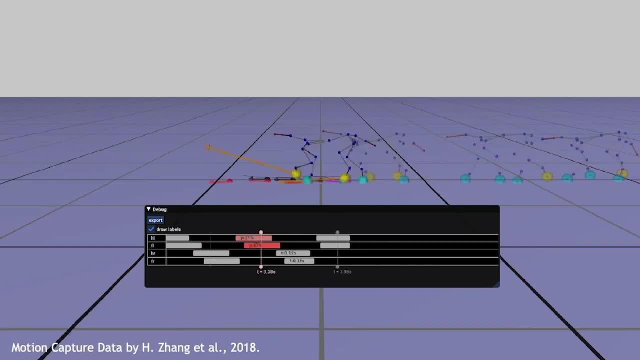 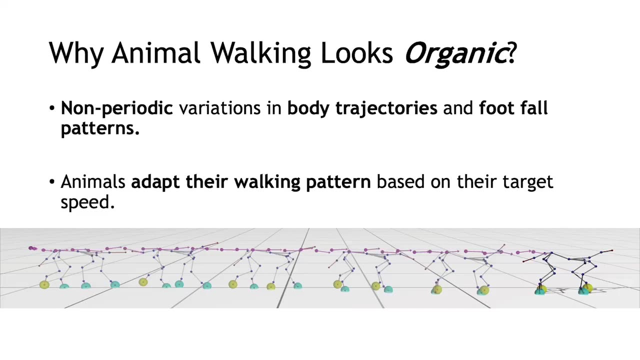 its footsteps are non-periodic and highly skewed. Finally, its body tends to shift or twist in sync with footsteps slightly. We want to reproduce the non-periodic nature of dogs' walking motions, specifically non-periodic footsteps, and the variation in body trajectories that makes their motions seem more organic. 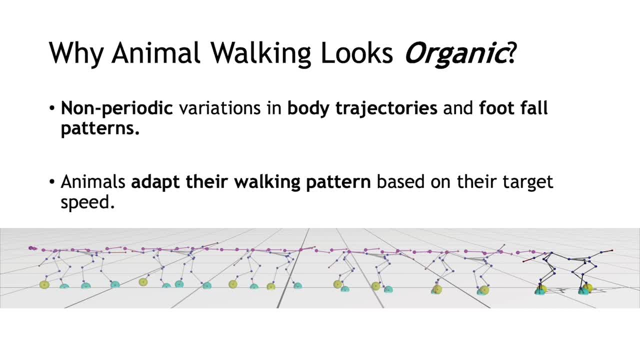 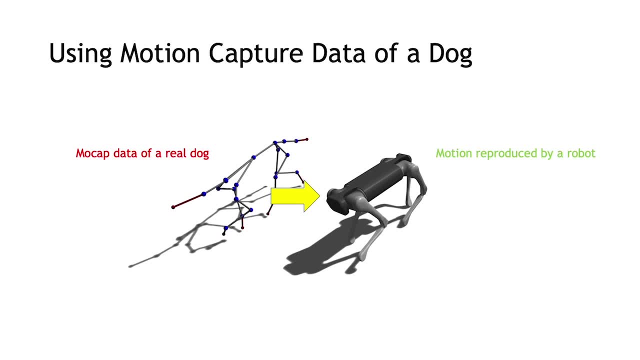 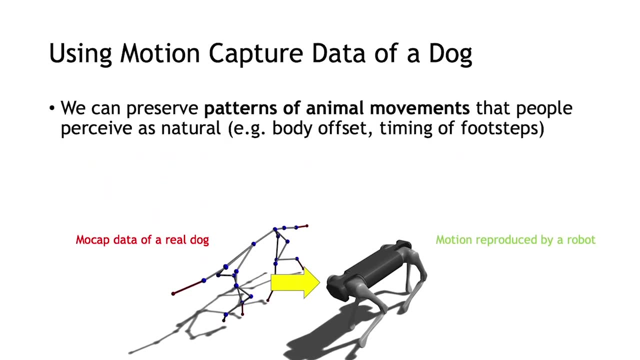 Moreover, we want to imitate the behavior of natural transitions between different gait patterns. In order to achieve this, we use motion capture data of a dog. This approach has too many ways to do. this has two main advantages. First, it preserves patterns of animal movements, such as body. 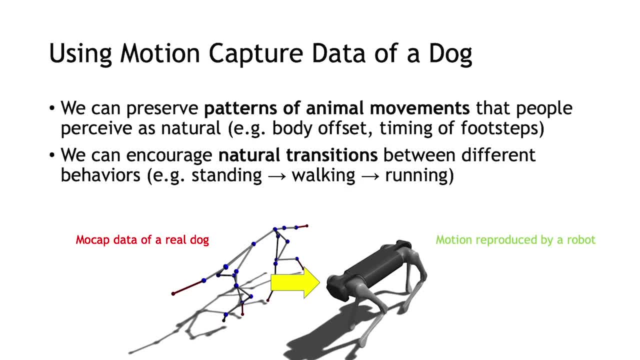 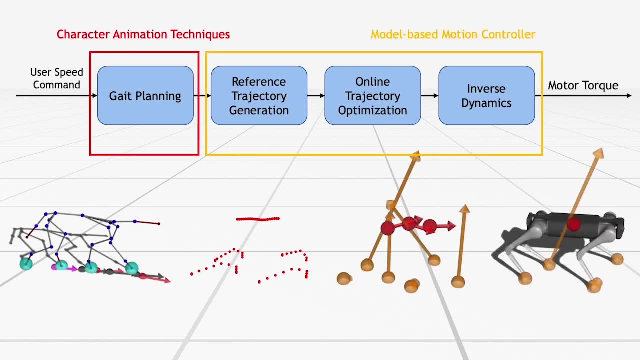 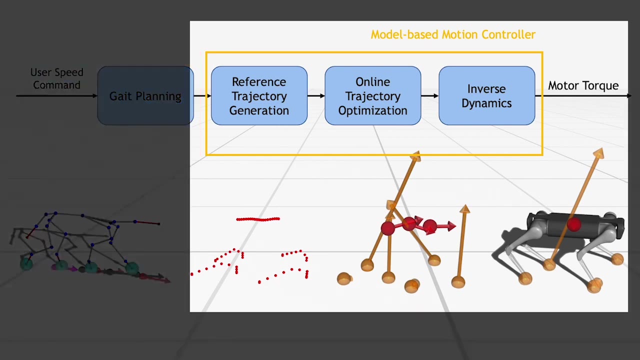 offset and timing of footsteps. Second, it encourages natural transitions between different behaviors without time-consuming and restrictive manual generation of transition animations, And we propose a control pipeline that combines character animation techniques with a state-of-the-art model-based motion controller architecture. Let me present the details of our model-based 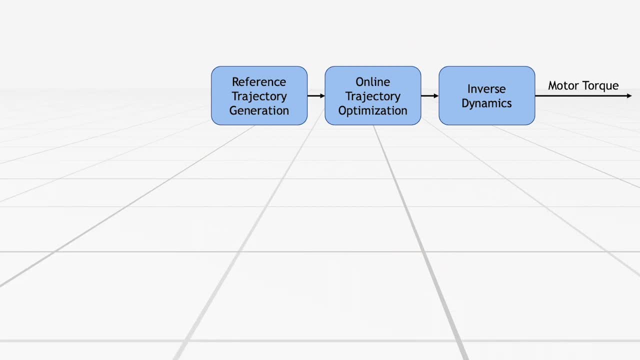 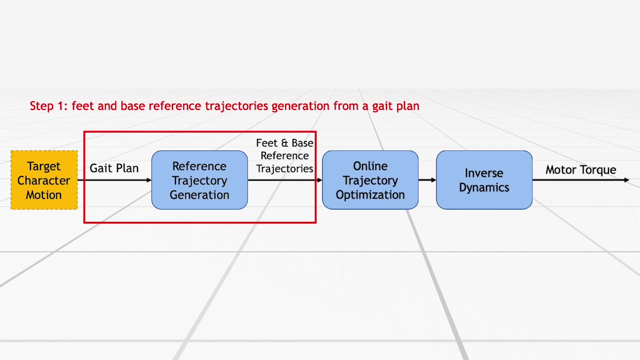 motion controller. first, Our motion controller reproduces a target-character motion clip on a robot. It extracts a gate plan from a target motion and generates motor torque commands. The first stage of the motion controller is reference trajectory generation. This stage takes a gate plan as an input and generates reference trajectories for the 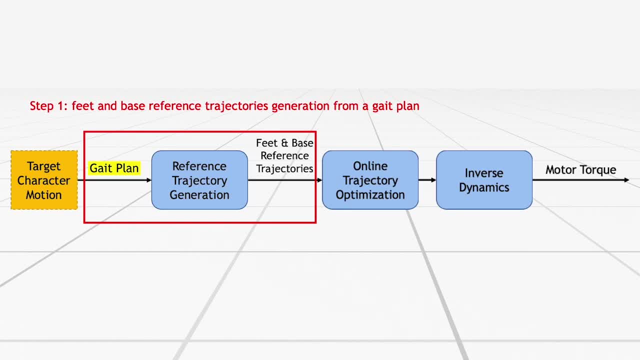 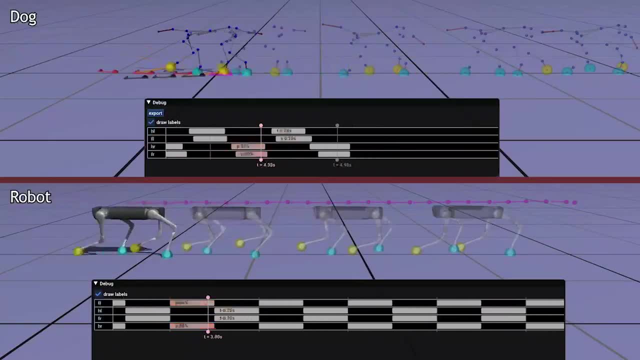 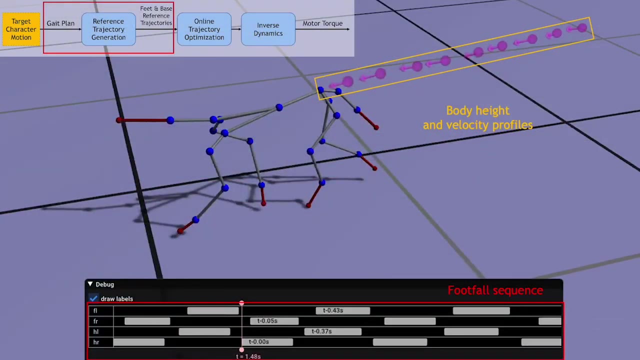 robot's base and feet. But what is the gate plan? I record that we aim to reproduce non-periodic footfall patterns and variations in body trajectory. Thus we extract a footfall sequence and body height and velocity profiles from a target dog motion and use this semantic information as a gate plan. 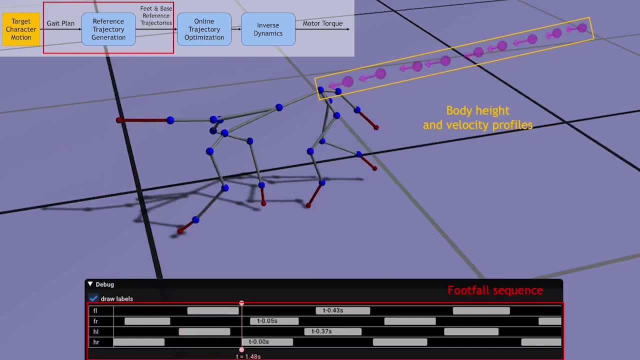 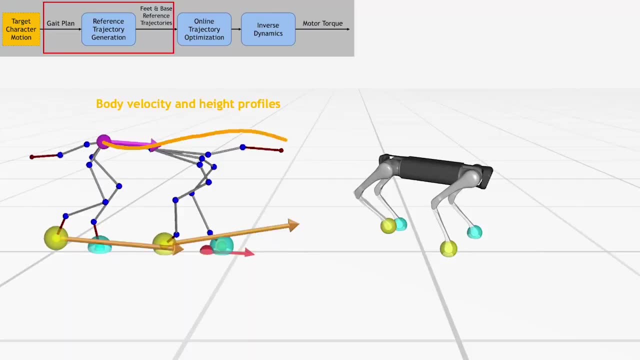 This approach allows us to transfer the dog motions to a robot with a different morphology and actuation power. We scale the speed and height profiles according to dimensions of the robot. Here we consider this scaling factor as a tuning parameter, as we found it to be intuitive and easy to. 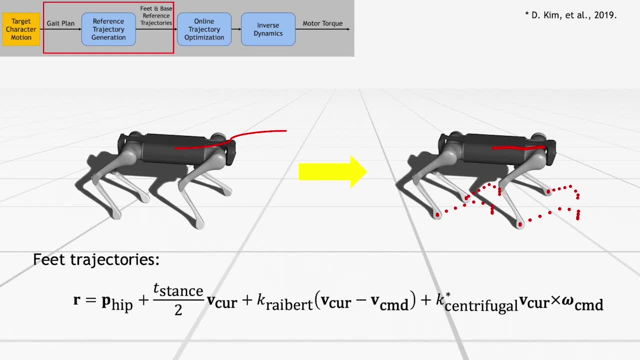 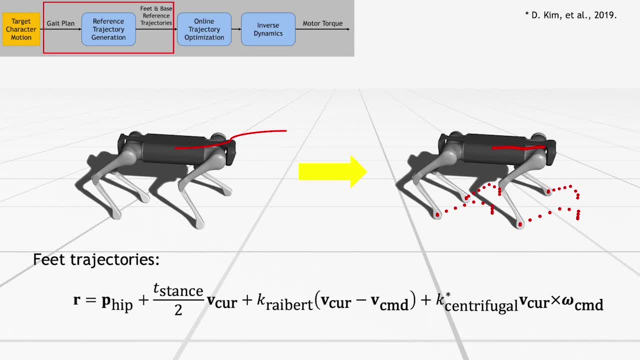 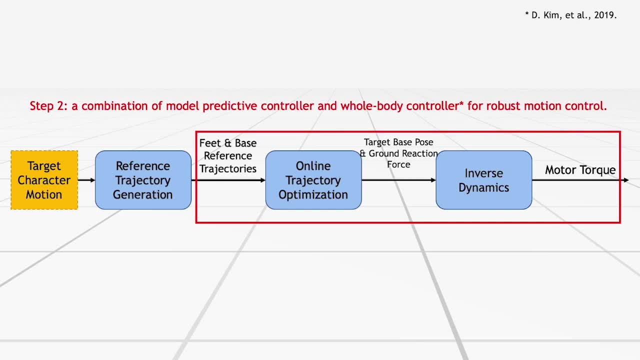 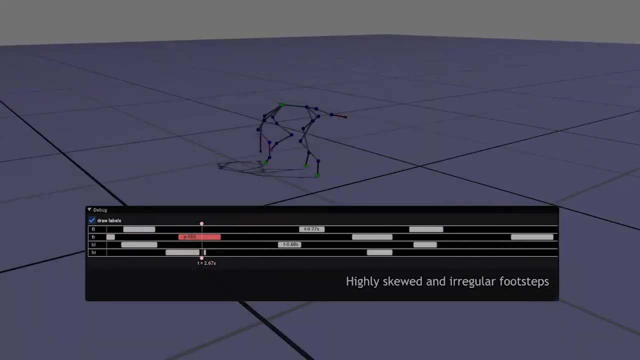 We then generate reference trajectories by a standard local motion trajectory planning strategy And then a combination of a model predictive controller and a whole body controller tracks the reference trajectories, mostly As a target gate plan extracted from motion capture. data may involve highly skewed, irregular footsteps and frequent non-contact phases. it can lead to poor performance in tracking. 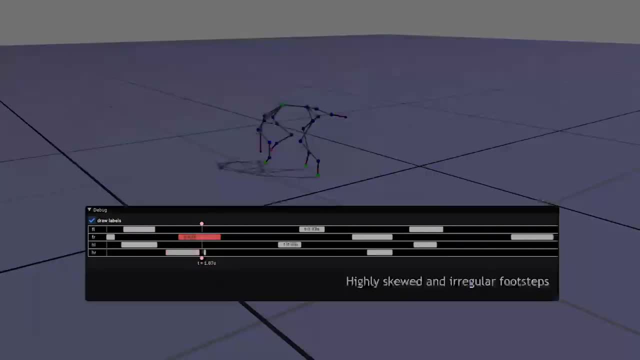 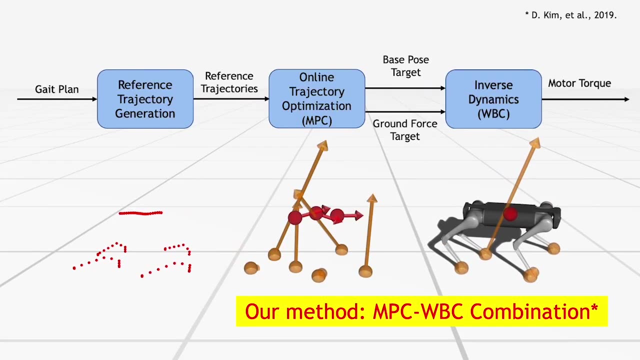 the base trajectory and cause the robot to lose control over the training, lose its balance and fall over. We therefore need a control stage that matches the input-deference trajectories as closely as possible, while ensuring that they remain feasible for the robot to track. To achieve this, we apply a combination of: 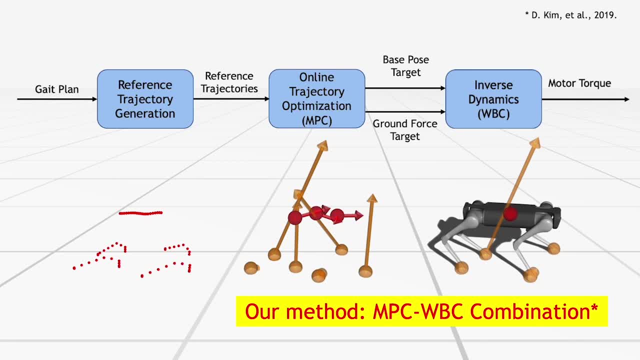 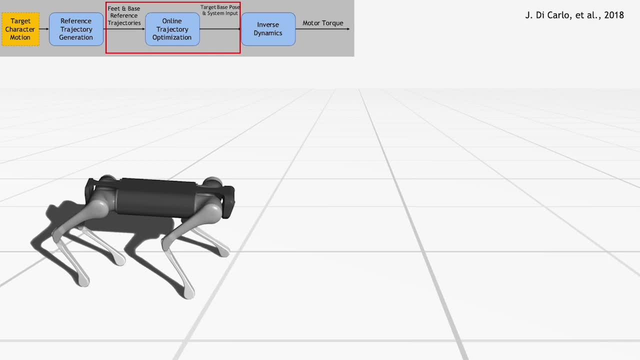 MPC and WBC in a similar manner as proposed by Kim et al. The MPC takes into account the dynamic effect aroused by movement and predicts the robot's behavior over a long time horizon. It leads to a more robust control execution that can handle underactuated configuration as well. Our MPC uses a simple lump-mass model that 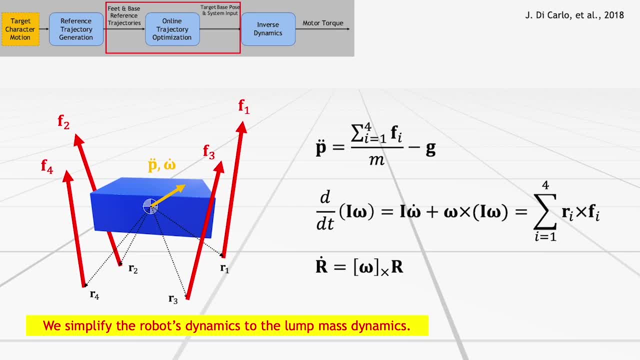 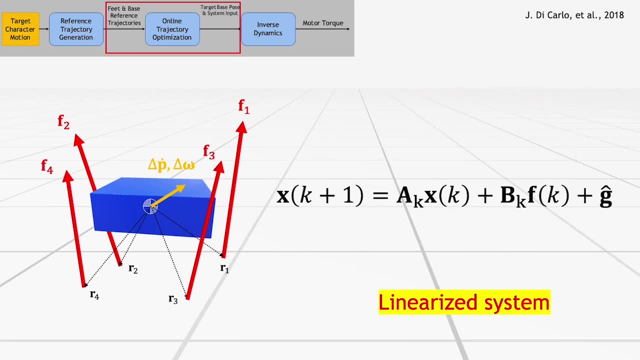 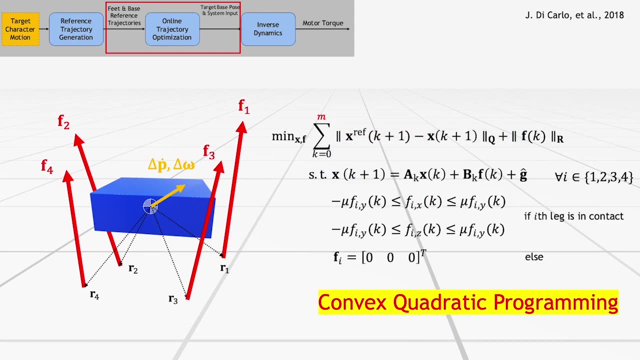 represents a robot as a 60-degree-of-freedom single-body object. We discretize and linearize the vacation of the motion and we forward-simulate multiple time steps with this simplified model. Then we find optimal ground reaction forces as well as body trajectory predictions that minimize trajectory error by solving a convex. 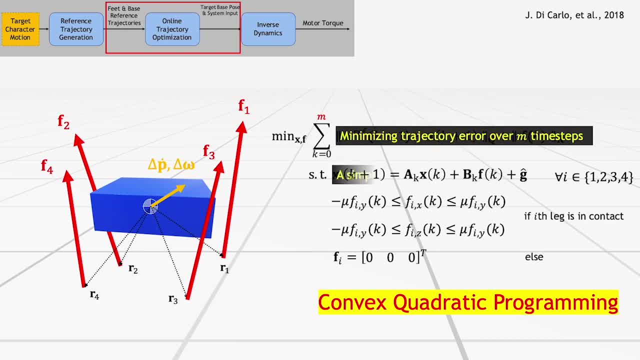 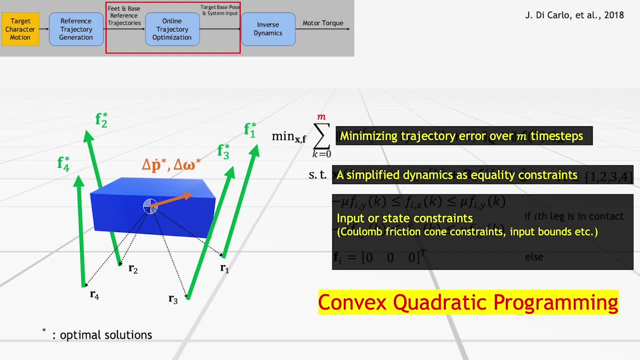 quadratic programming. The problem is to minimize sum of trajectory error over multiple time steps subject to the linearized dynamics and input and state of motion. The problem is to minimize sum of trajectory error over multiple time steps subject to the linearized dynamics and input-and-state. 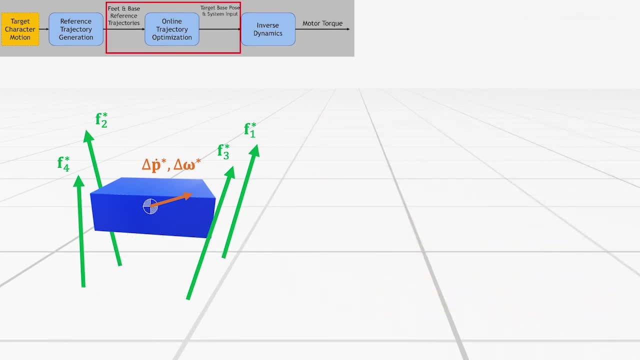 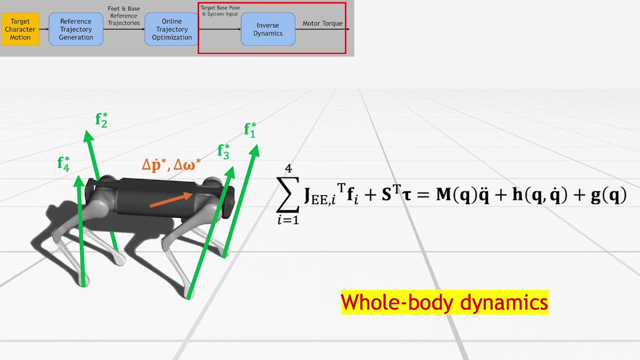 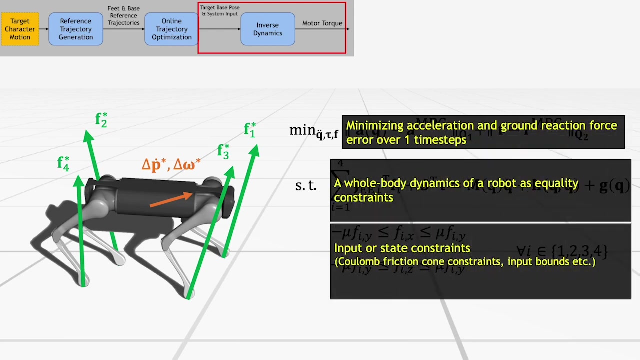 constraints. As our final step, we track this ground reaction force target and the long-time horizon optimal trajectory, while taking into account whole-body dynamics. We use a whole-body control method. It finds joint torque commands that allow robot to follow trajectory predictions from MPC by solving another convex quadratic program. In summary, we can see that the robot is able to control the whole-body dynamics of the whole-body control method. We can also see that the robot is able to control the whole-body control method. We can also see that the robot is able to control the whole-body control method. 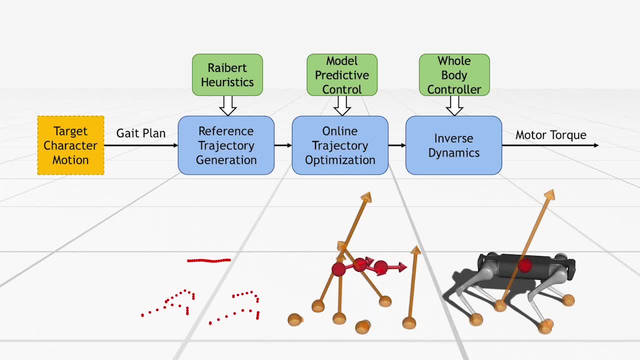 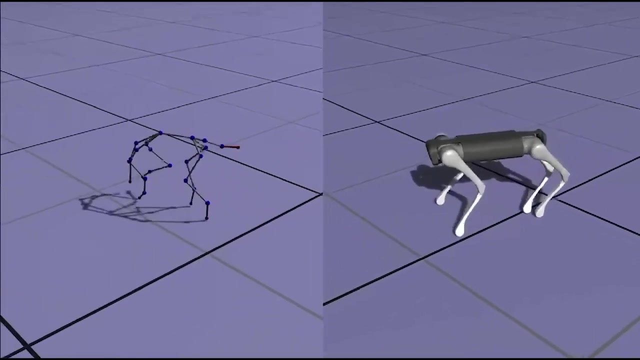 In summary, we use a motion controller that consists of three stages: From a gate plane extracted from a motion clip, we generate kinematic reference trajectory and convert it to dynamics-aware trajectories with MPC And finally we compute joint torque to follow the MPC trajectory. This control stack can successfully transfer a target dog motion. 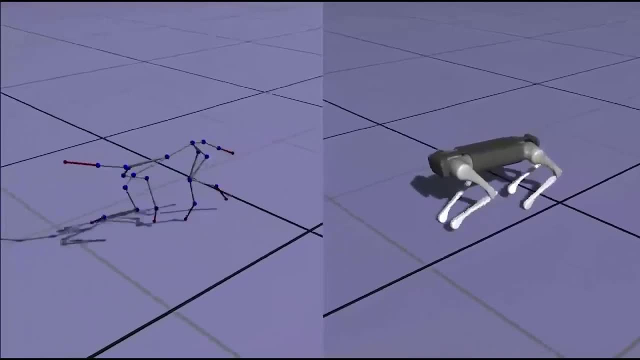 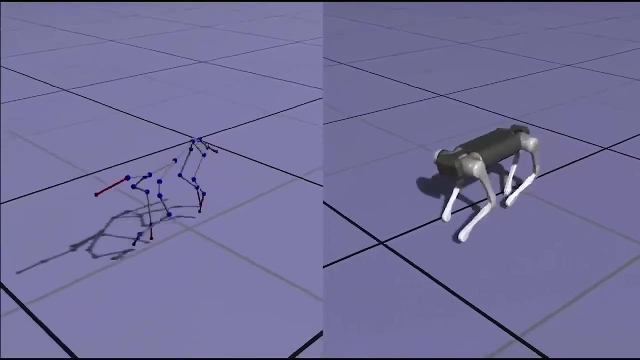 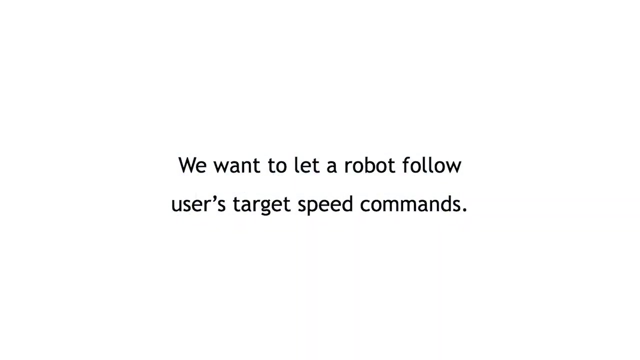 to a quadrupedal robot. As you can see in these video clips, the robot motion replicates small body movements and non-periodic footsteps of animal motions. The motion controller can generate the motion given a gate plan extracted from a motion clip. 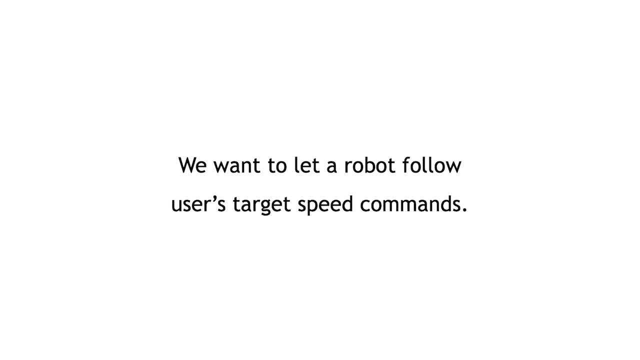 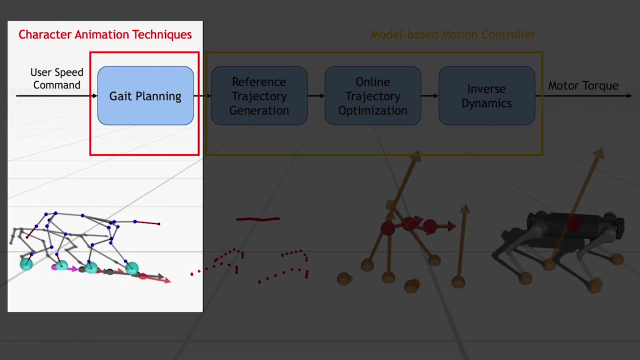 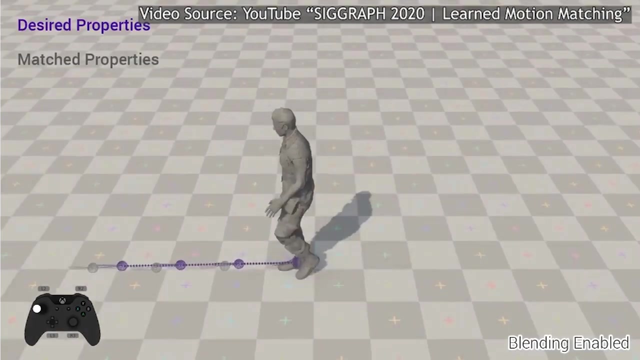 But we want to let a robot follow a user's target speed command. For this purpose, we apply a data-driven computer animation tool that generates a target motion based on a high-level command, such as a desired moving speed and a turning rate. More specifically, we use a character animation method called motion matching. 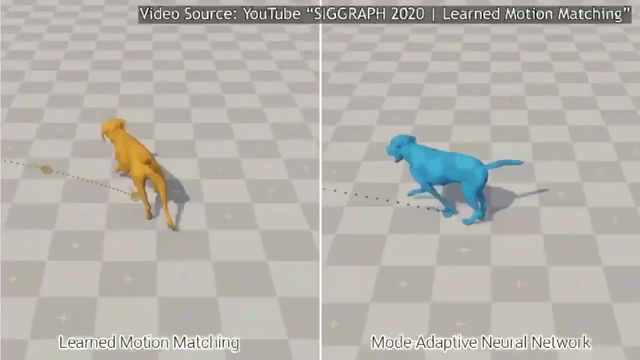 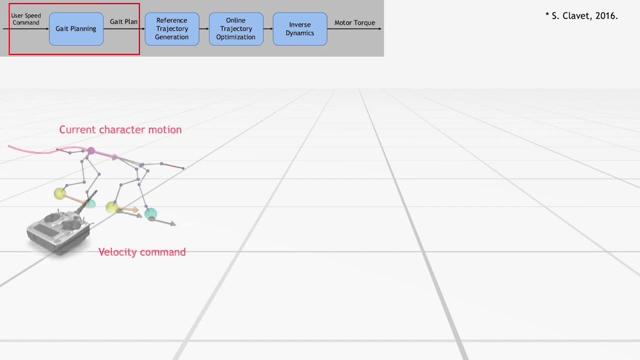 This method generates motion sequences that is responsive to a user's command. The idea of motion matching is simple. Given the current state of some predefined motion features and the user's target input, we retrieve the best sequence to play from the huge mocap dataset. 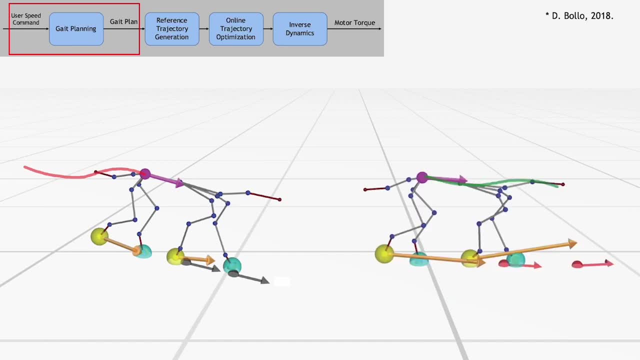 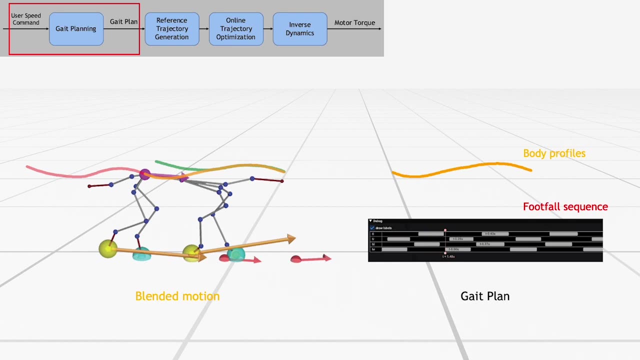 And we blend the retrieved motion into the currently played motion sequence And from there we extract the footfall sequence by freshly holding the feet velocity and feet height of the character And also we extract the balance of motion. This is the body velocity and height profile. 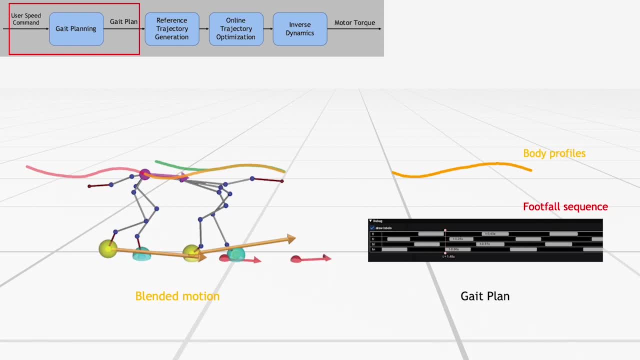 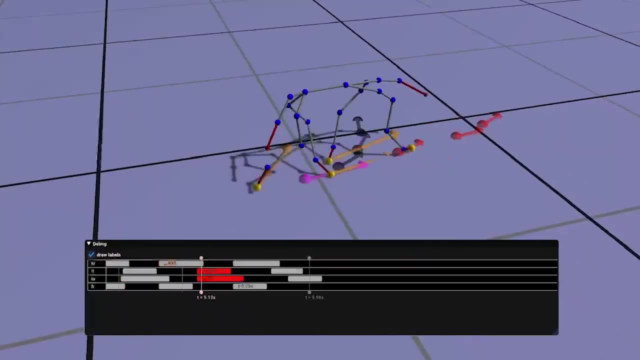 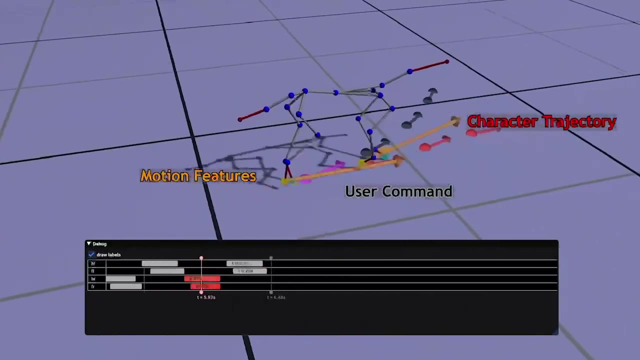 As already mentioned, this semantic information is used as a gate plan. So let's see how well motion matching works. In this video you can see our quadrupedal character follows the user's command responsibly. We can also notice that the footfall sequence extracted from the motion sequence is also reasonable. 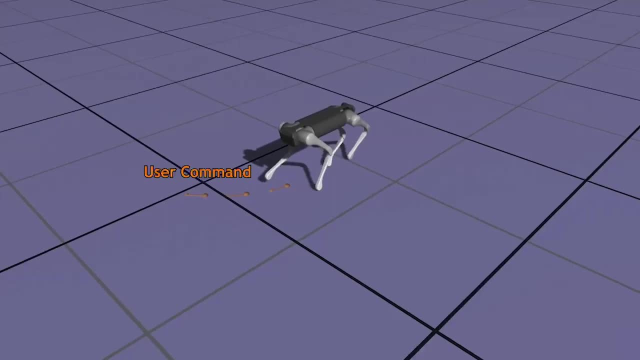 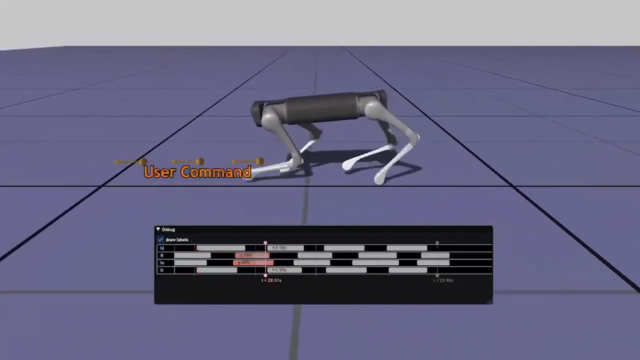 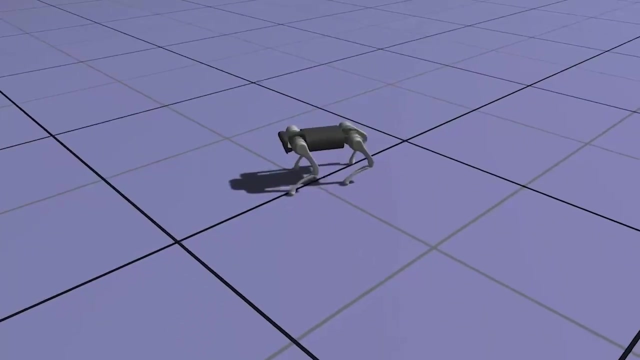 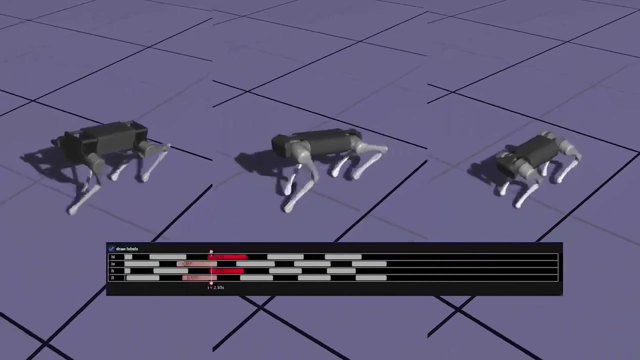 And all together we can let a robot follow the user's command and walk in an animal-like style. We can apply our pipeline to various robotic platforms. The only parameter that needs to be tuned for a specific robot model is the scaling factor that is used to transfer the character motions from the dataset to the robot. 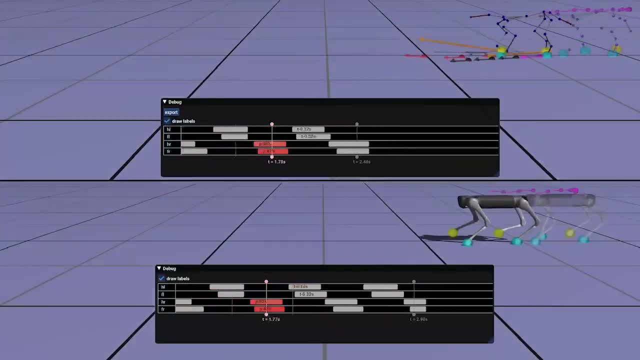 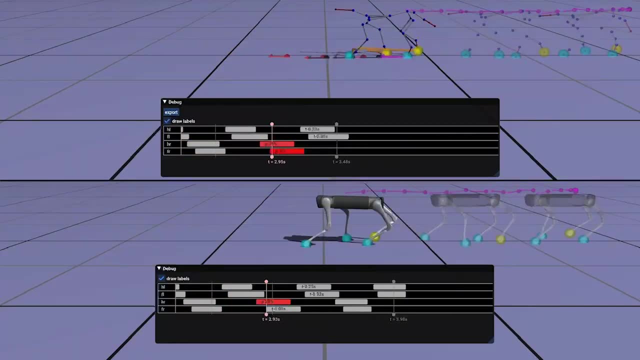 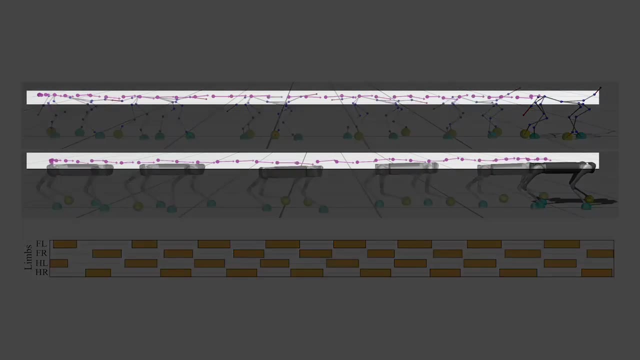 We evaluated the efficacy of our control pipeline with two scenarios. In the first scenario, constant forward speed command of 0.8 m per second was given And, as I highlighted, the robot can replicate the small variations in body movements that we observe in animal motions. 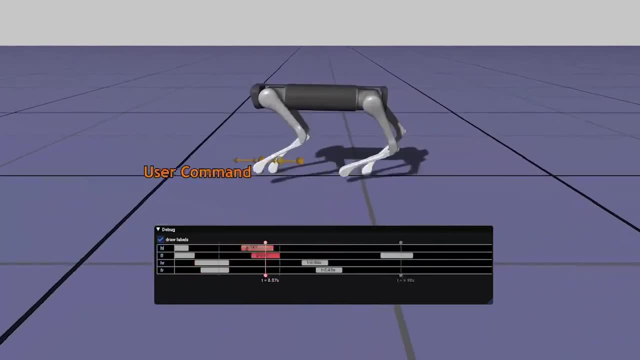 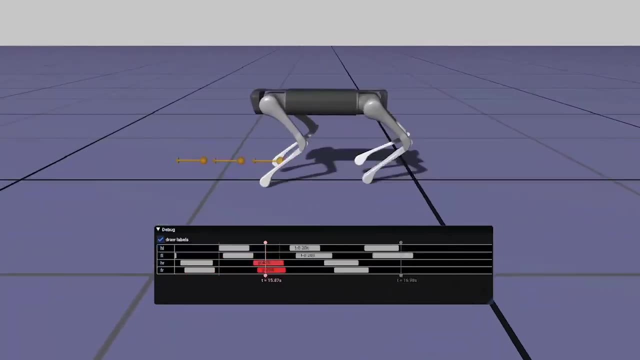 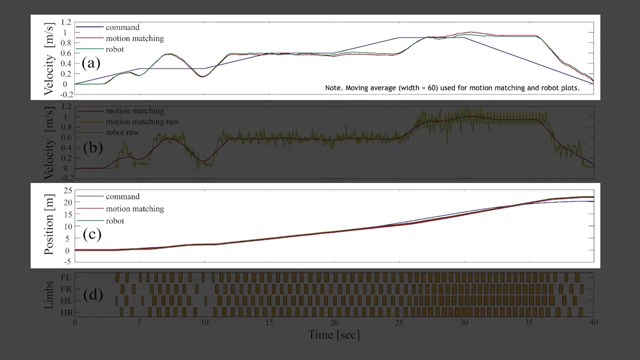 In the second scenario a forward speed command was varied over a range between 0 to 0.9 m per second. The plots here show that the robot is able to track the user's command inputs. There are some mismatches and delays in comparison to the target command in velocity level. 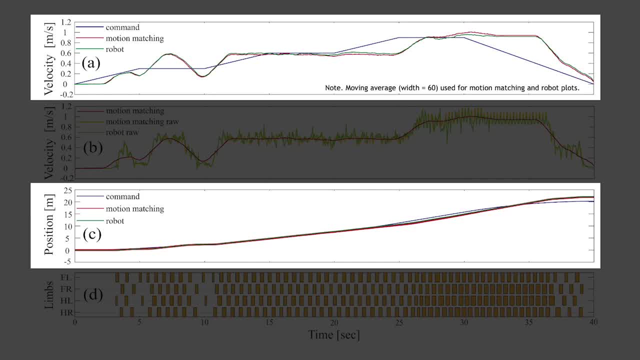 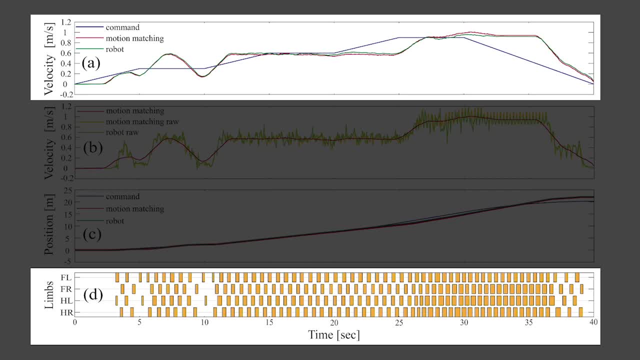 but overall the target-based position discerning from the velocity command can still be tracked reasonably well. The footfall sequence of the robot is depicted in the last row. It is visible that the robot swiftly changes its gait based on the target-based speed. 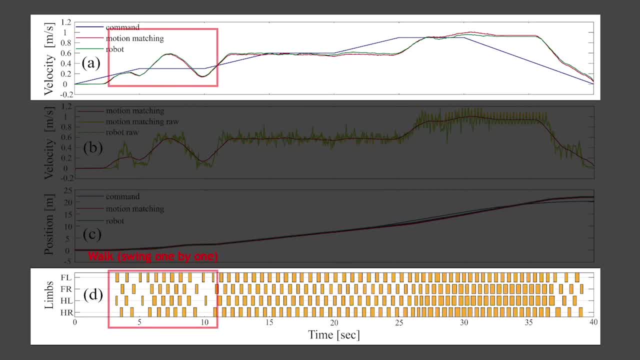 In the range of 0 to 0.3 m per second, the gait planner generates a slow walking gait that moves the robot's feet one by one As the command speed increases. when the command speed increases to 0.3 to 0.6 m per second, 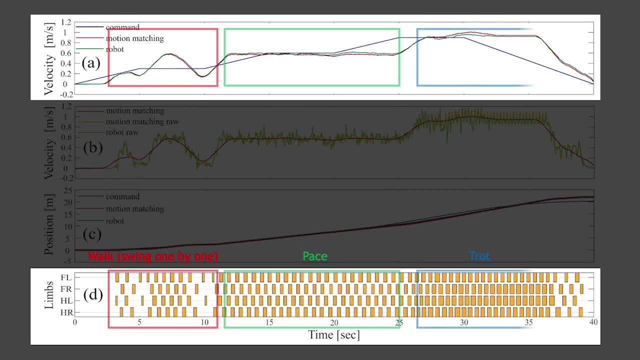 the gait is changed to a pace gait And in the range of 0.6 to 0.9, the gait is changed to a torque gait. We can see that the footfall frequency as well as the duration ratio of swing to stance phases. 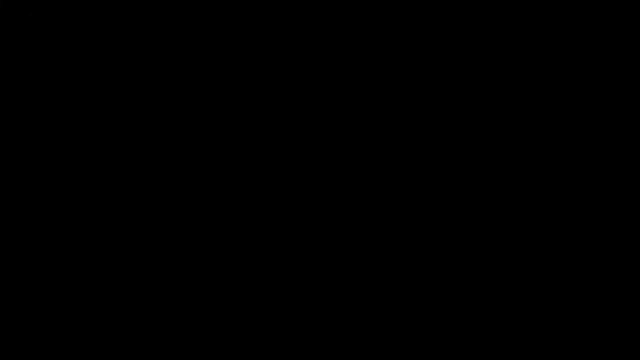 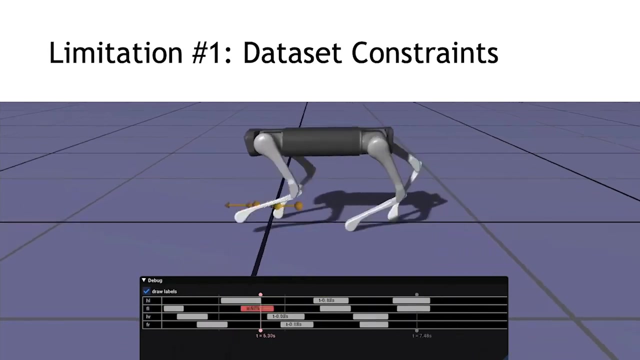 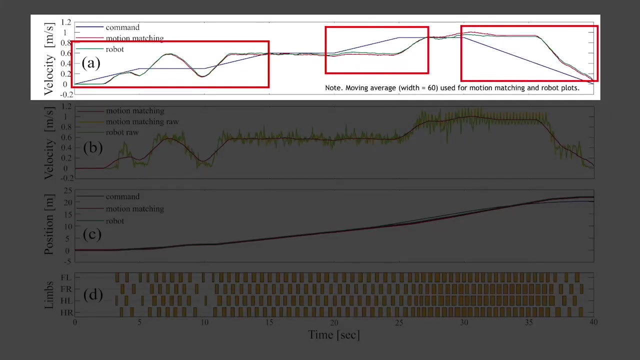 are increased with higher speed commands. After experiments, our method revealed two main limitations. First, since motion matching simply searches through the existing dataset, the discerning robot motions are limited by the richness of the motion capture dataset. This results in mismatches and delays in a robot's velocity.